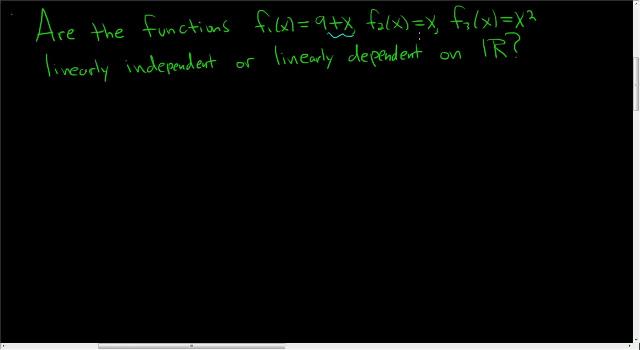 We're being asked if the functions 9 plus x, x and x squared are linearly independent or linearly dependent on the set of real numbers. Solution: We'll start by supposing we have what's called a linear combination of our three functions and that it's equal to zero. So 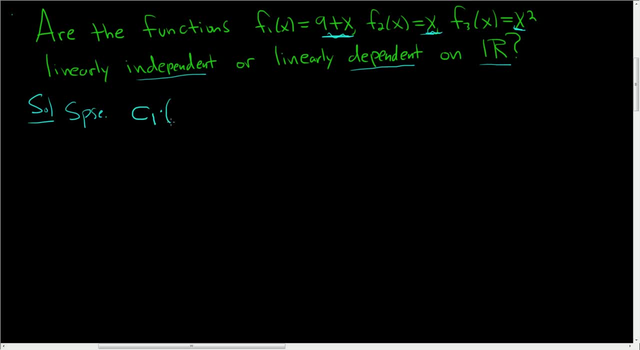 what is a linear combination? Well, it's c sub 1 times 9 plus x. Here c sub 1 is a number, plus c sub 2 times x, plus c sub 3 times x squared, And we suppose that this is equal to. 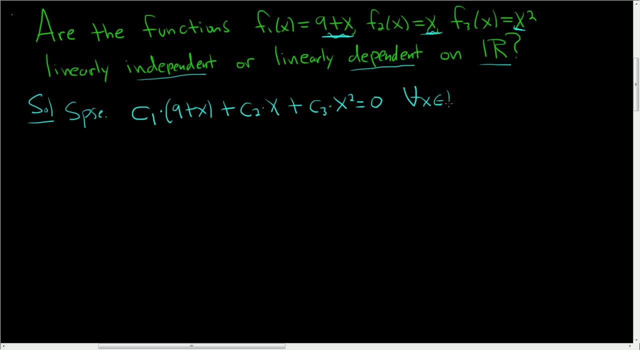 zero for all x in the set of real numbers and some arbitrary c sub 1, c sub 2, c sub 3, and r. One of two things will happen at this point: All of these c sub i's, c sub 1, c sub 2, c sub 3- will be equal to zero. So all c sub i are equal to zero. If this is true, 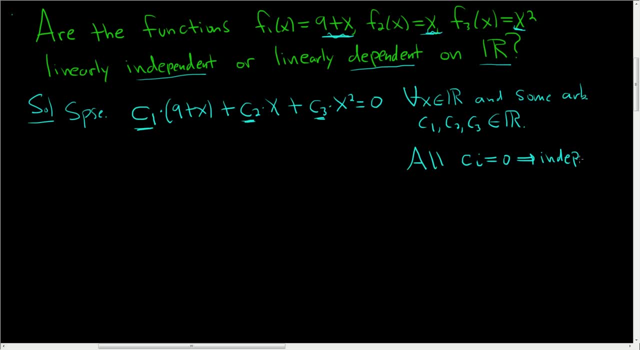 then the answer is independent Or not. all c sub i are zero. If this is true, then the answer is dependent. Okay, so we continue. So we distribute 9 c sub 1 plus x squared, We're going to have a linear combination of our three functions. We're going to: 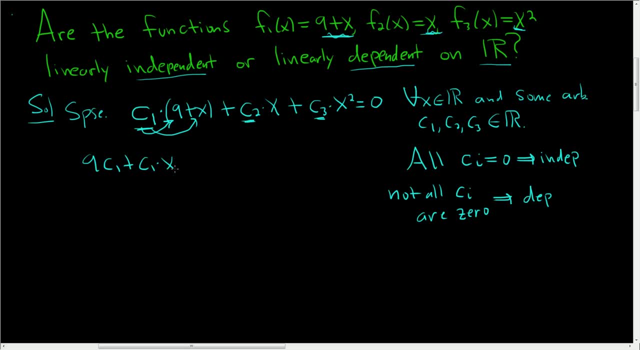 plus c sub 1x plus c sub 2x plus c sub 3 times x. squared, We set this equal to 0.. At this point we collect like terms, So 9 c sub 1 plus c sub 1 plus c sub 2 times x. 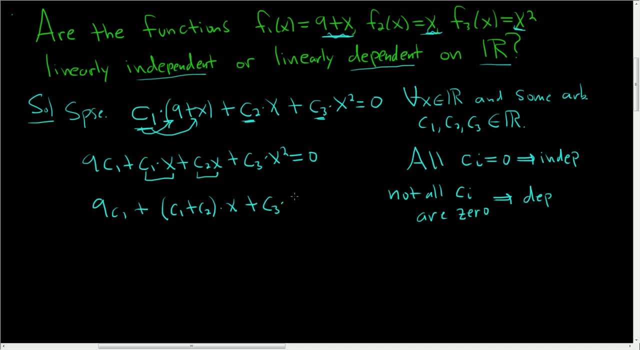 plus c sub 3 times x squared, and this is equal to 0.. So how do we figure out what the c's are? Well, the left-hand side is a polynomial. The right-hand side is a polynomial. Two polynomials are equal only. 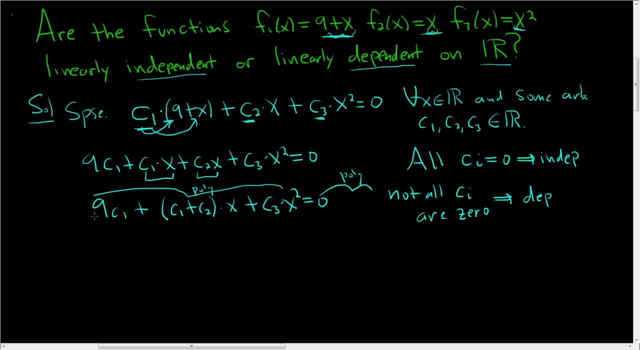 when their coefficients are the same. So we'll start by what's called equating coefficients. So first let's look at the constant term. This is 9 c sub 1, and this is equal to the constant term over here, which is 0.